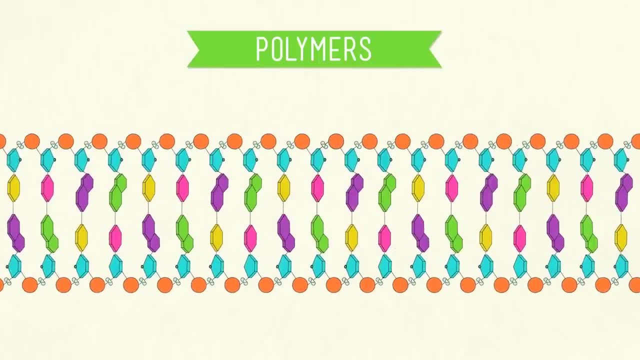 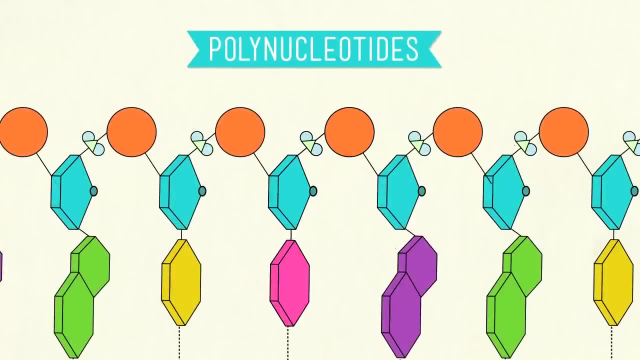 Structurally they're polymers, which means that each one is made up of many small repeating molecules. In DNA, these small units are called nucleotides. Link them together and you have yourself a polynucleotide. Now, before we actually put these tiny parts together to build a DNA molecule, 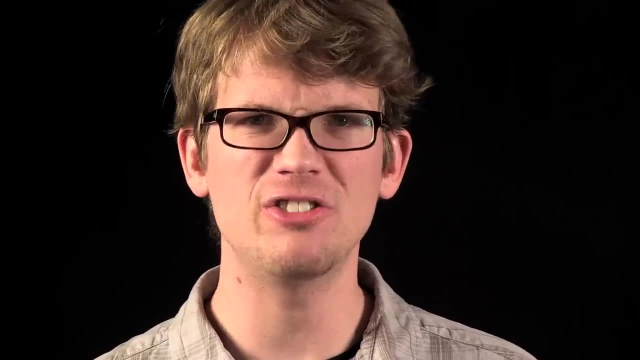 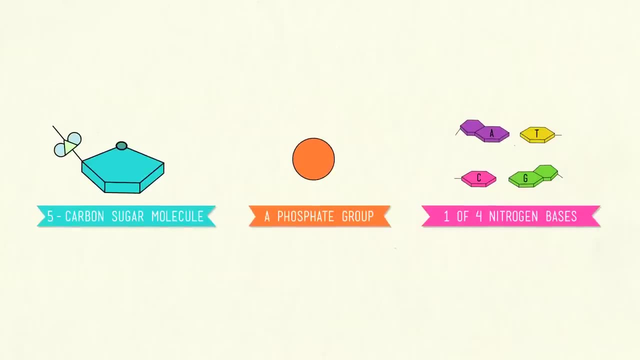 like some microscopic piece of Ikea furniture. let's first take a look at what makes up each nucleotide. We're gonna need three things: One, a five carbon sugar molecule. Two, a phosphate group. And three, one of four nitrogen bases. 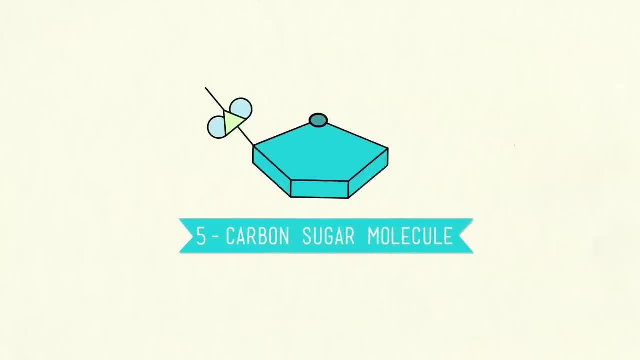 DNA gets the first part of its name from our first ingredient, the sugar molecule, which is called deoxyribose. But all the really significant stuff, the genetic coding that makes you you, is found among the four nitrogenous bases: adenine, thymine, cytosine and guanine. 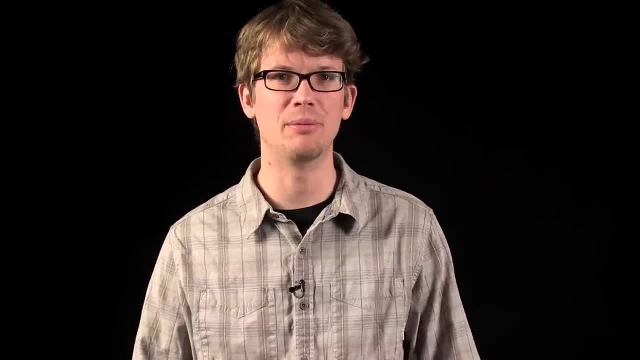 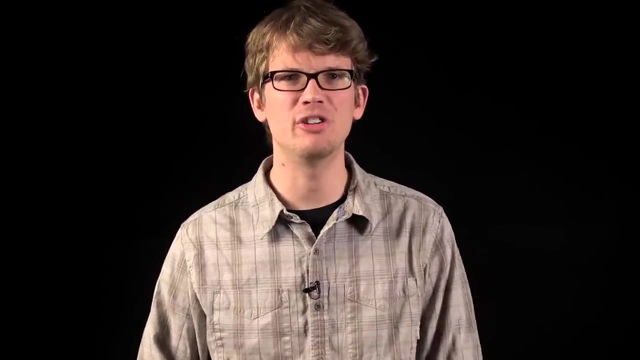 It's important to note that in living organisms, DNA doesn't exist as a single polynucleotide molecule, but rather a pair of molecules that are held tightly together. They're like an intertwined, microscopic double spiral staircase: Basically just a ladder, but twisted. 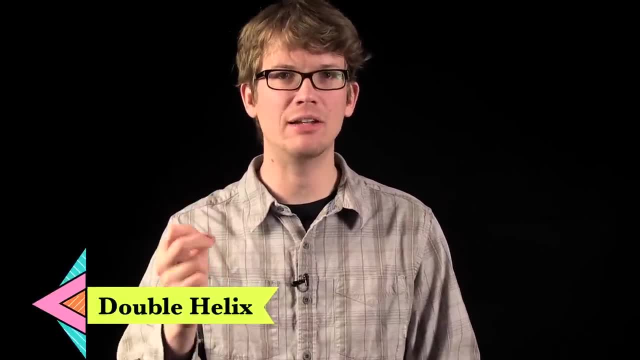 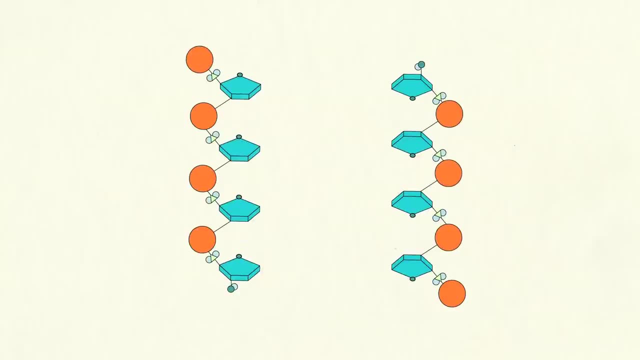 The famous double helix And, like any good structure, we have to have a main support. In DNA, the sugars and phosphates bond together to form twin backbones. These sugar phosphate bonds run down each side of the helix, but chemically in opposite directions. 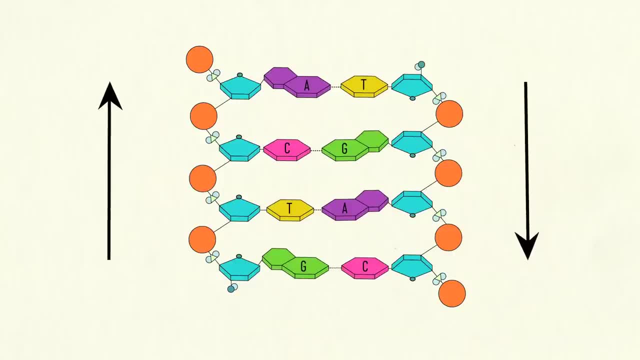 In other words, if you look at each of the sugar phosphate backbones, you'll see that one appears to be upside down in relation to the other. One strand begins at the top of the first phosphate connected to the sugar molecule's fifth carbon. 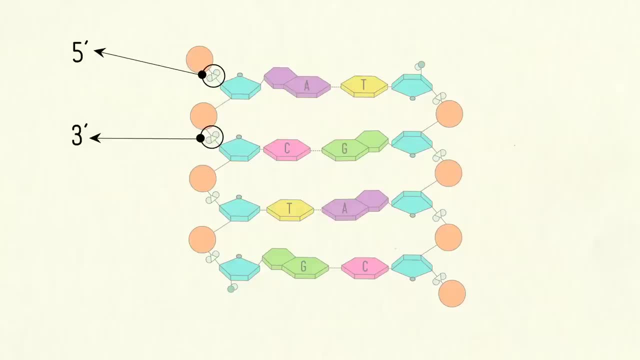 and then ending where the next phosphate would go, with a free end at the sugar's third carbon. This creates a pattern called five prime and three prime. I've always thought that deoxyribose with an arrow with the oxygen as a point. 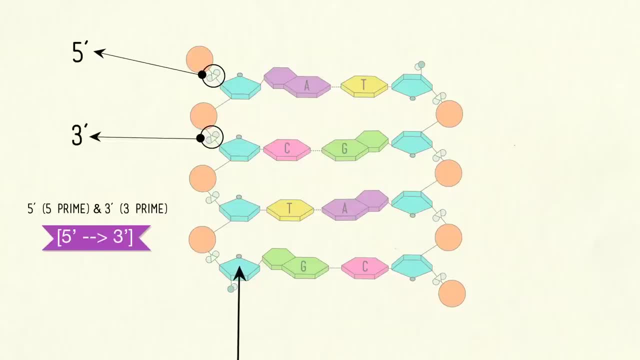 it always points from three prime to five prime. Now, on the other strand, it's exactly the opposite. It begins up top with a free end at the sugar's third carbon, and then the phosphates connect to the sugar's fifth carbons all the way down. 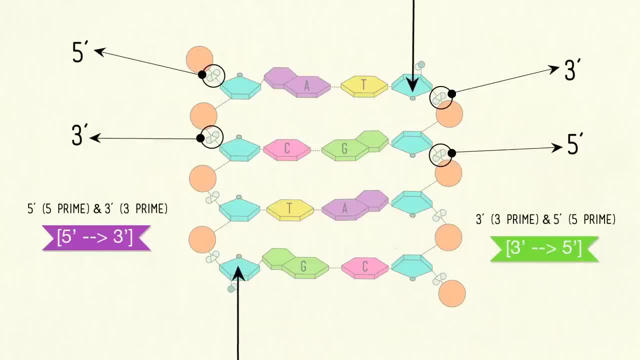 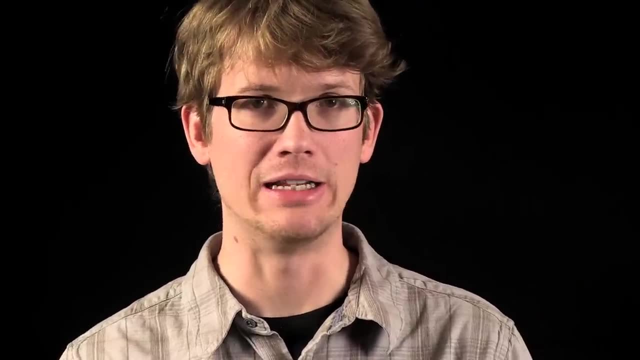 And it ends at the bottom with the phosphate, and you've probably figured this out already, but this is called the three prime to five prime direction. Now it is time to make ourselves one of these famous double helices. These two long chains are linked together by the nitrogenous bases. 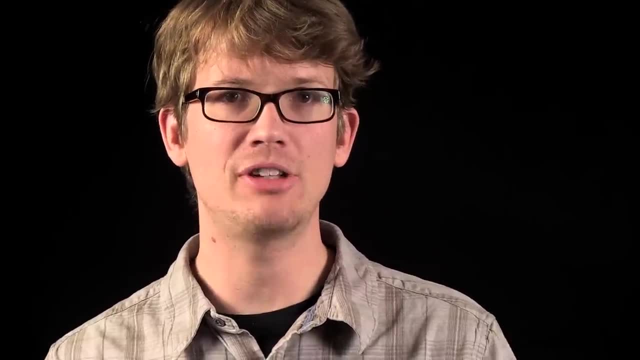 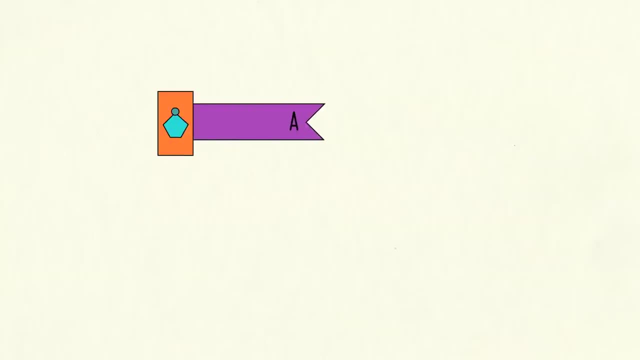 via relatively weak hydrogen bonds, But they can't be just any pair of nitrogenous bases, Thankfully. when it comes to figuring out what part goes where, all you have to do is remember that if one nucleotide has an adenine base, only thymine can be its counterpart. 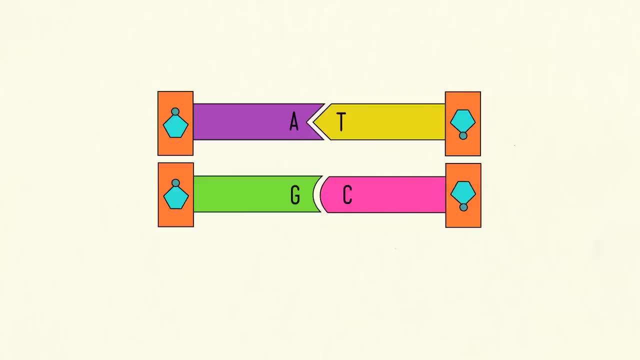 Likewise, guanine can only bond with cytosine. These bonded nitrogenous bases are called base pairs. The G-C pairing has three hydrogen bonds, making it slightly stronger than the A-T base pair, which only has two. It's the order of these four nucleobases. 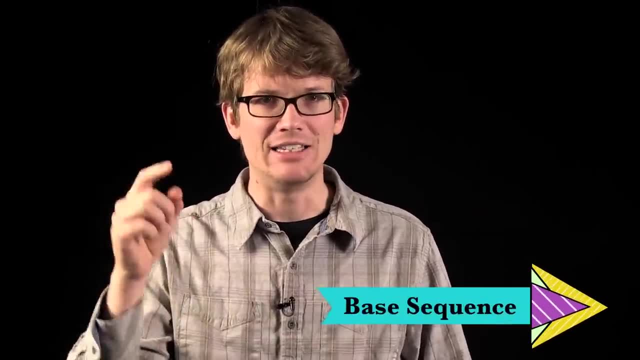 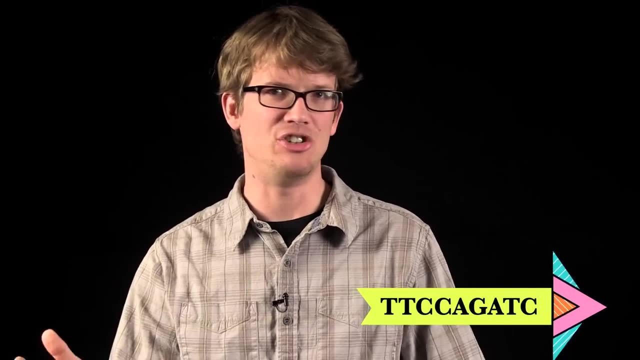 or the base sequence that allows your DNA to create you. So A-G-G-T-C-C-A-T-G means something completely different as a base sequence than, say, T-T-C-A-G-T-C. Human chromosome 1, the largest of all of our chromosomes. 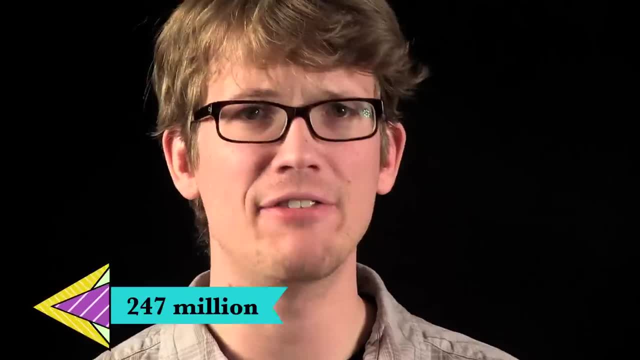 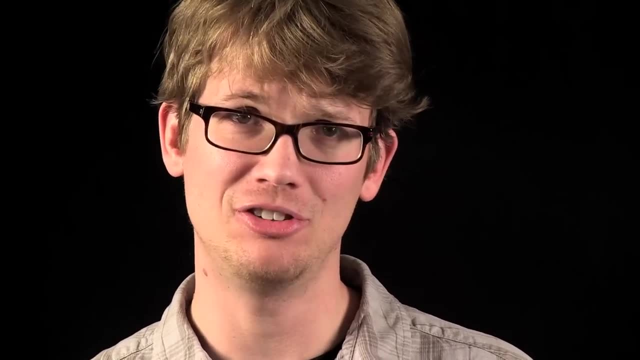 contains a single molecule of DNA with 247 million base pairs. If you printed all of the letters of chromosome 1 into a book, it would be about 200,000 pages long, And each of your somatic cells has 46 DNA molecules tightly packed into its nucleus. 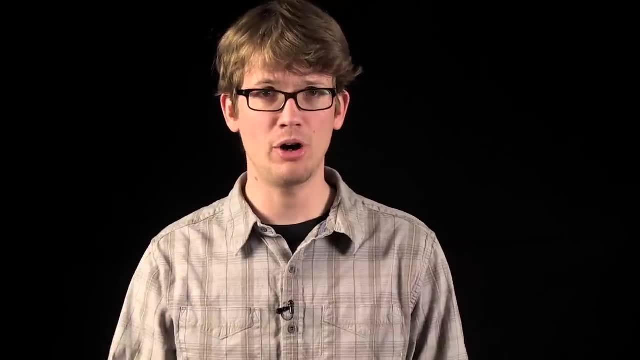 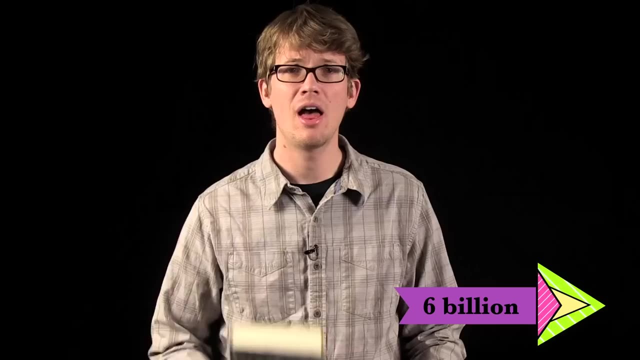 That's one for each of your chromosomes. Put all 46 molecules together and we're talking about roughly 6 billion base pairs in every cell. This is the longest book that I've ever read. It's about 1,000 pages long. 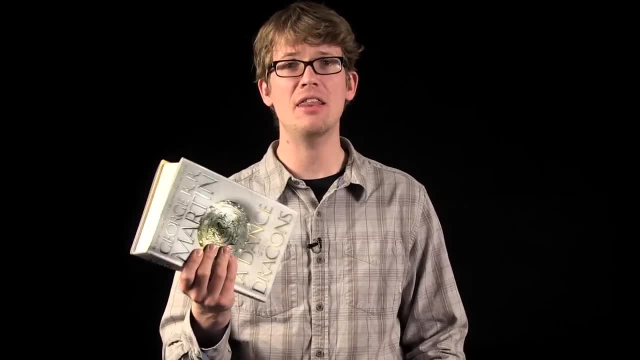 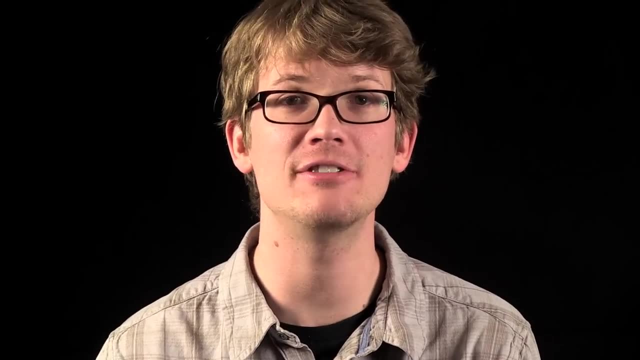 If we were to fill it with our DNA sequence, we'd need about 10,000 of them to fit our entire genome. Pop quiz: Let's test your skills using a very short strand of DNA. I'll give you one base sequence. 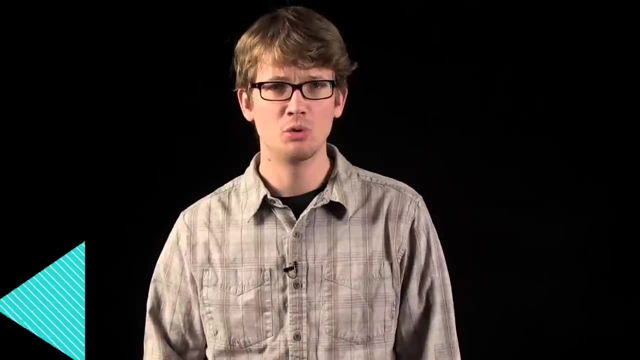 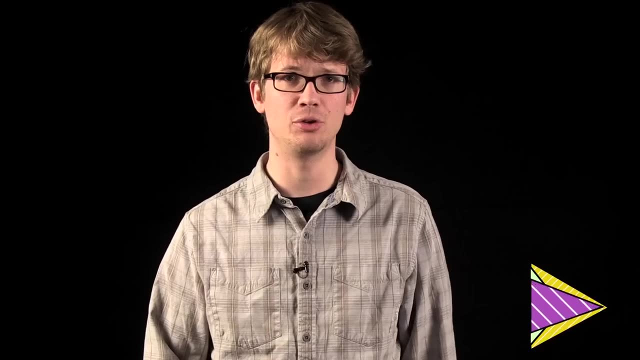 You give me the base sequence that appears on the other strand. Okay, here goes. So we've got a 5 prime A-G-G-T-C-C-G to 3 prime and, time's up, The answer is 3 prime T-C-C-A-T-G. 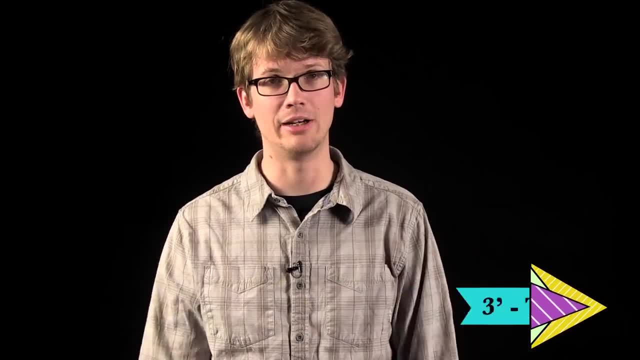 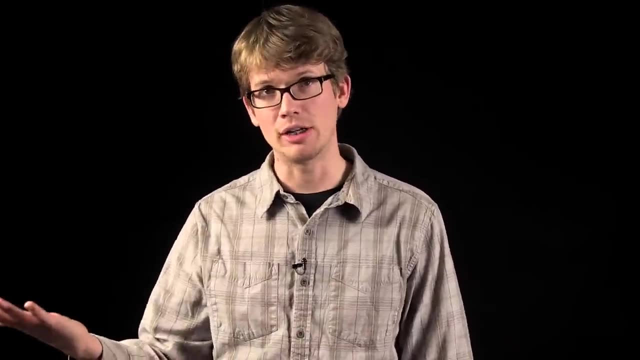 See how that works. It's not super complicated. Since each nitrogenous base only has one counterpart, you can use one base sequence to predict what its matching sequence is going to look like. So could I make the same base sequence with a strand of that other nucleic acid RNA? 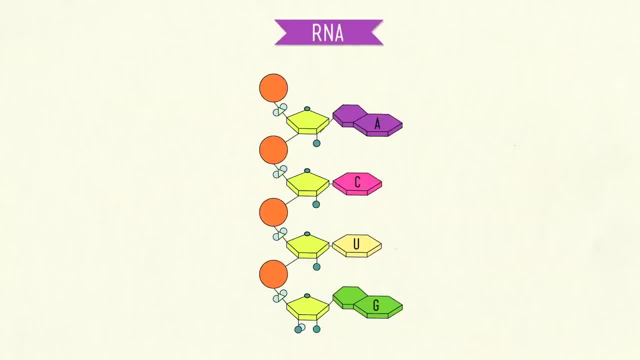 No, you could not. RNA is certainly similar to its cousin DNA. It has a sugar phosphate backbone with nucleotide bases attached to it. But there are three major differences. One: RNA is a single-stranded molecule, No double helix here. 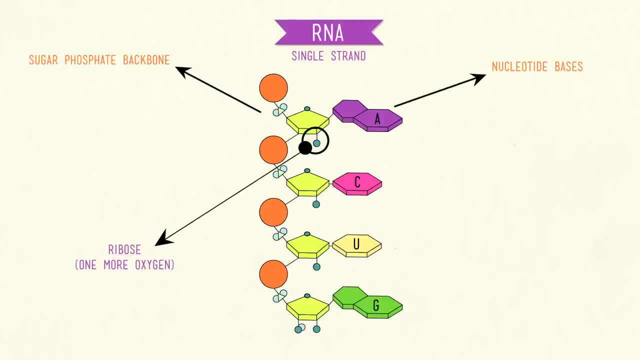 Two, the sugar in RNA is ribose, which has one more oxygen atom than deoxyribose. hence the whole starting with an R instead of a D thing. And finally, RNA does not contain thymine. Its fourth nucleotide is the base uracil. 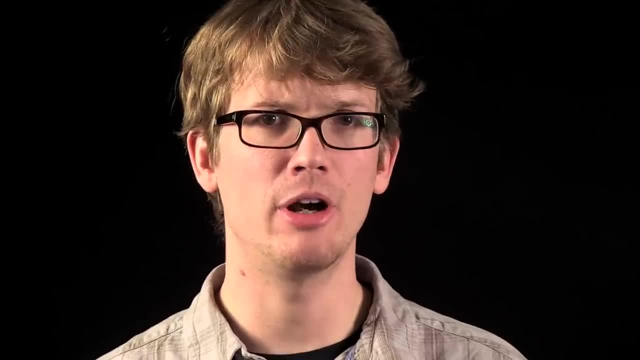 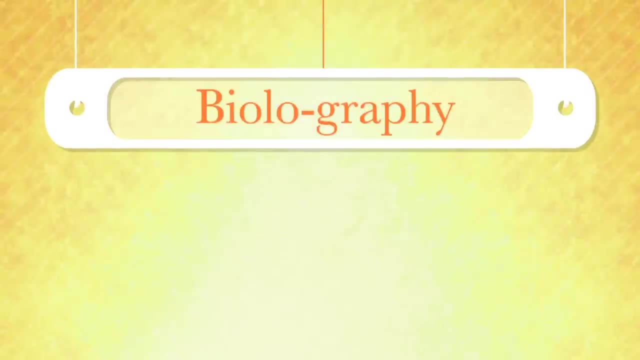 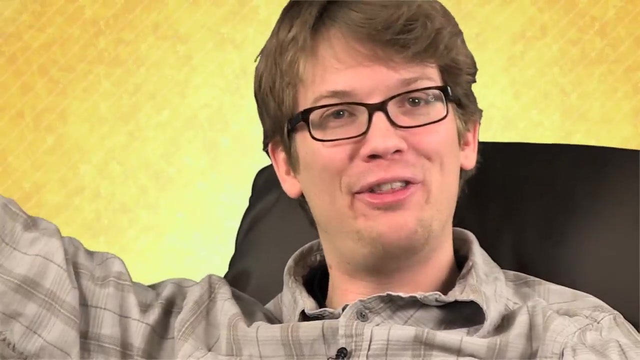 so it bonds with adenine instead. RNA is super important to the production of our proteins and you'll see later that it has a crucial role in the replication of DNA. But first Biographies. Yes, plural this week, because when you start talking about something, 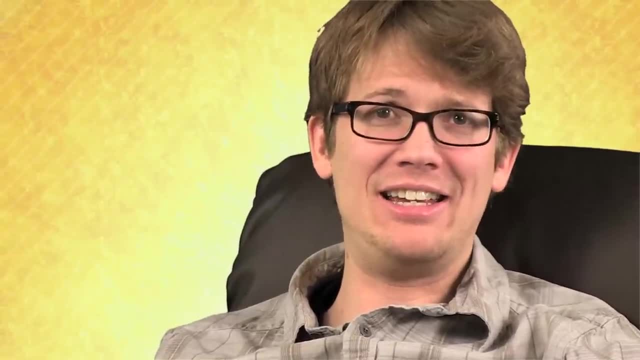 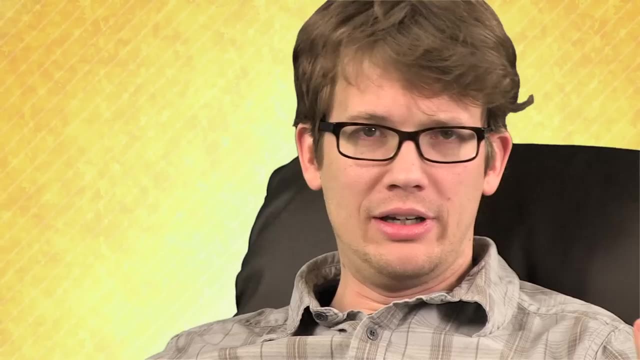 as multitudinously awesome and elegant as DNA. you have to wonder just who figured all this stuff out and how big was their brain? Well, unsurprisingly, it actually took a lot of different brains in a lot of different countries and nearly a hundred years of thinking to do it. 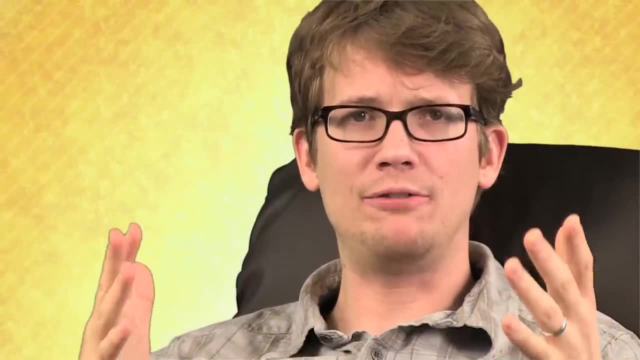 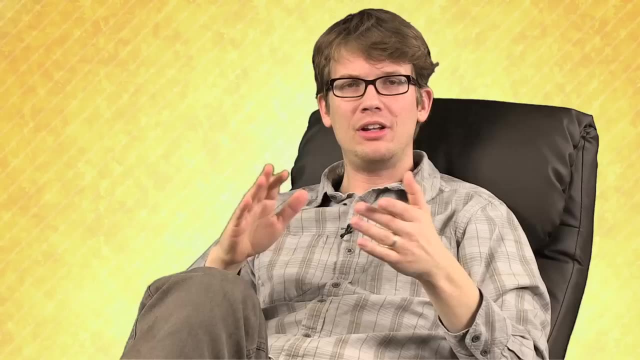 The names you usually hear when someone asks who discovered DNA are James Watson and Francis Crick. but that's bunk. They did not discover DNA, nor did they discover that DNA contained genetic information. DNA itself was discovered in 1869 by a Swiss biologist named Friedrich Mieschack. 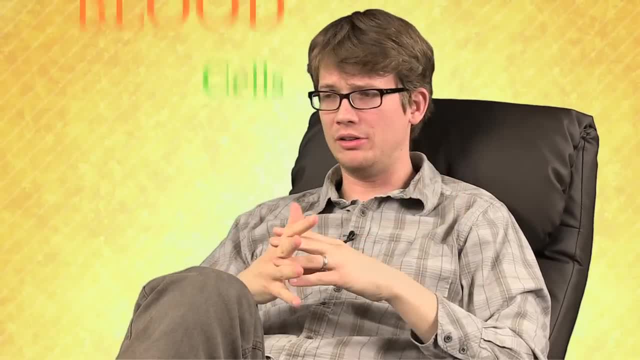 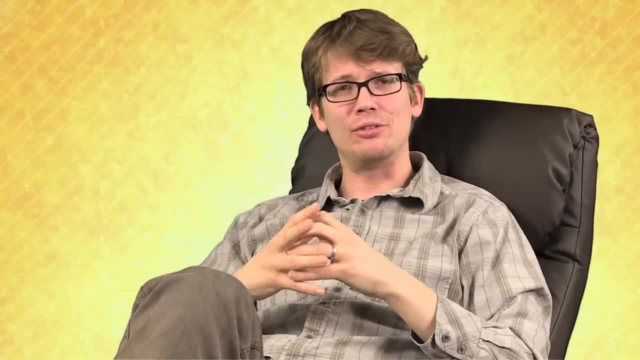 His deal was studying white blood cells and he got those white blood cells in the most horrible way you could possibly imagine, from collecting used bandages from a nearby hospital. For science he did it: He bathed the cells in warm alcohol to remove the lipids. 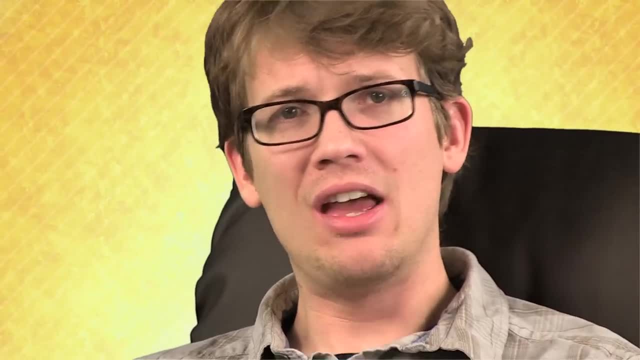 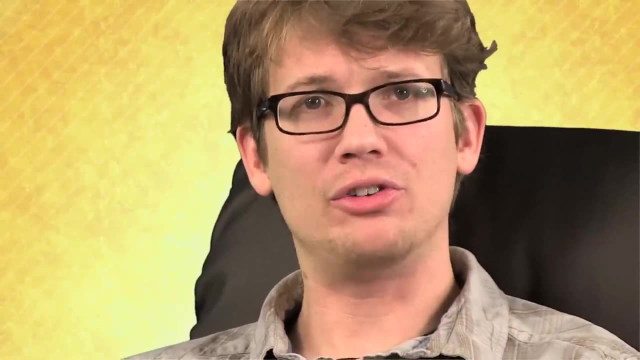 and then he set enzymes loose on them to digest the proteins, and what was left after all of that was this snotty, gray stuff that he knew must be some new kind of biological substance. He called it nuclein, what was later to become known as nucleic acid. 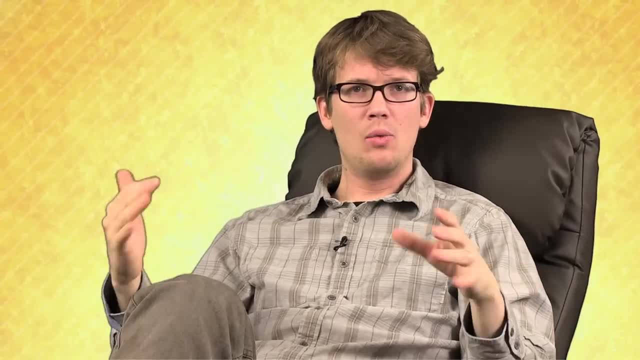 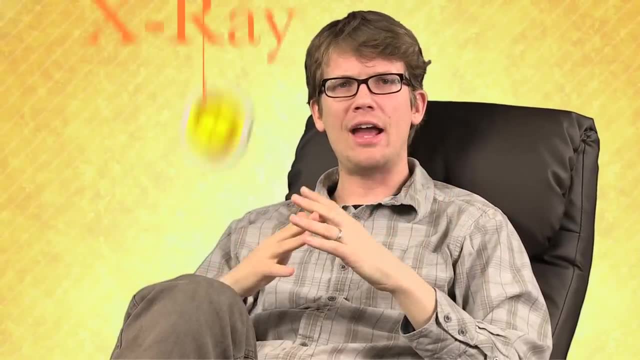 So Mieschack didn't know what its role was or what it looked like. One of the scientists who helped figure that out was Rosalind Franklin, a young biophysicist in London, nearly a hundred years later, Using a technique called X-ray diffraction. 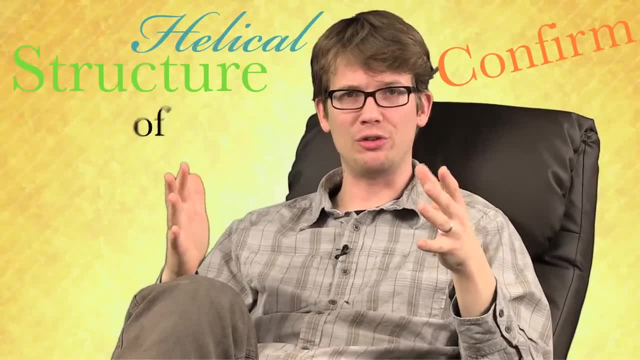 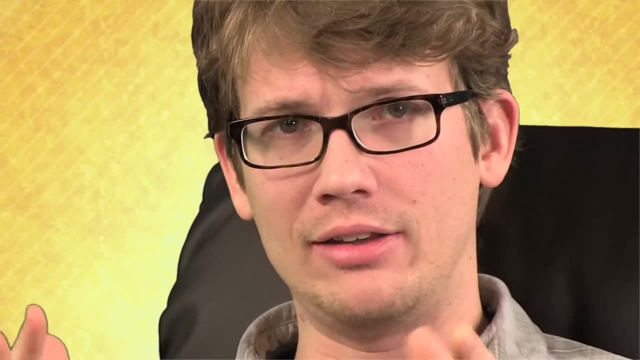 Franklin may have been the first to confirm the helical structure of DNA. She also figured out that the sugar phosphate backbone existed on the outside of the structure. So why is Rosalind Franklin not exactly a household name? Well, two reasons. One, unlike Watson and Crick. 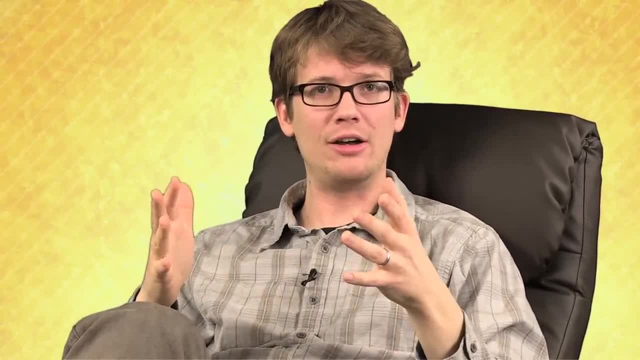 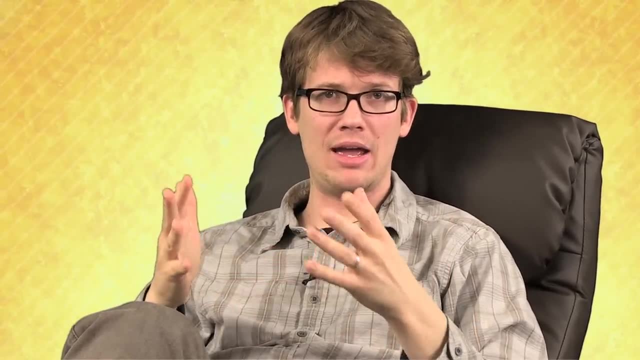 Franklin was happy to share data with her rivals. It was Franklin who informed Watson and Crick that an earlier theory of a triple helix structure was not possible, And in doing so she indicated that DNA may indeed be a double helix. Later, her remedies confirming the helical structure of DNA. 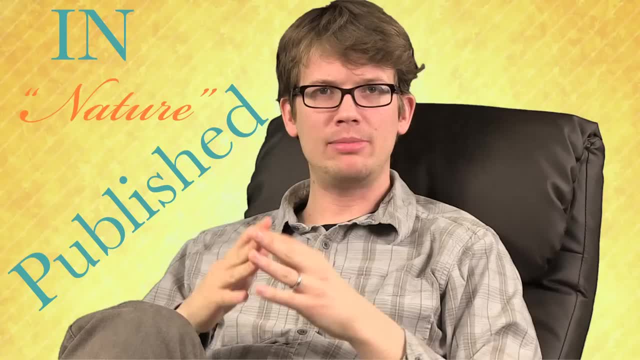 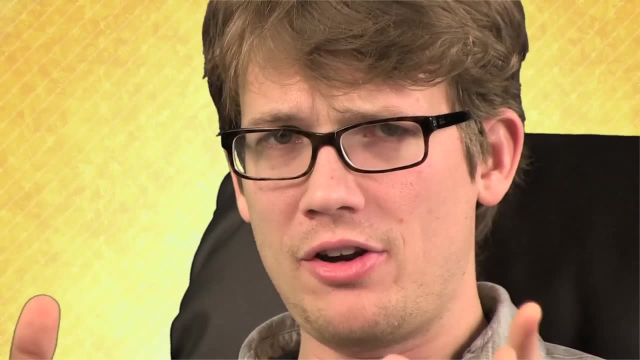 were shown to Watson without her knowledge. Her work was eventually published in Nature, but not until after two papers by Watson and Crick had already appeared, in which the duo only hinted at her contribution. Even worse than that, the Nobel Prize Committee couldn't even consider her. 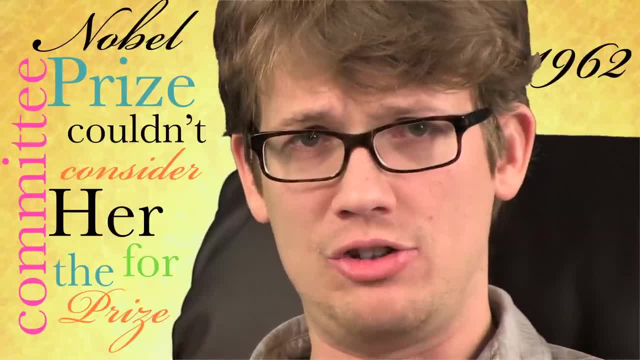 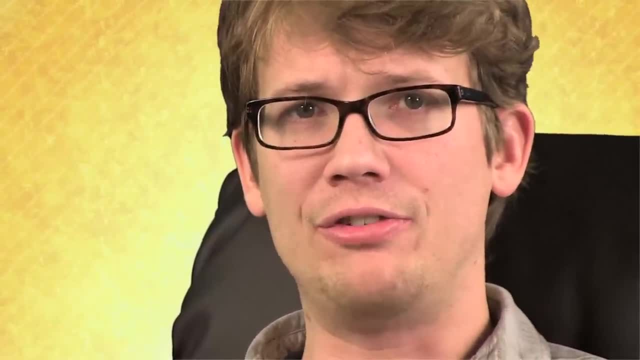 for the prize that they awarded in 1962 because of how dead she was. The really tragic thing is that it's totally possible that her scientific work may have led to her early death of ovarian cancer at the age of 37. At the time, the X-ray diffraction technology 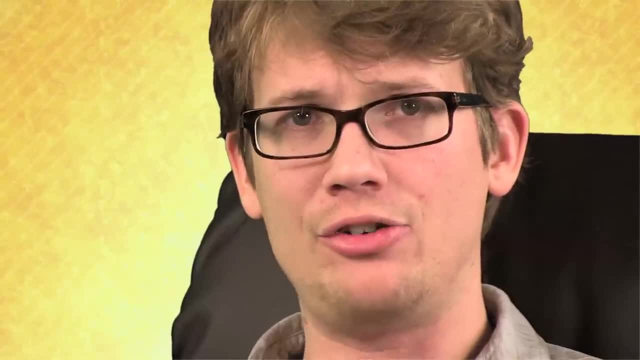 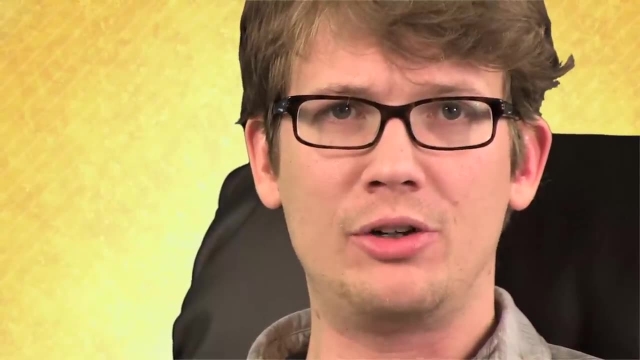 that she was using to photograph DNA required dangerous amounts of radiation exposure, and Franklin rarely took precautions to protect herself. Nobel Prizes cannot be awarded posthumously. Many believe that she would have shared Watson and Crick's medal if she had been alive to receive it. 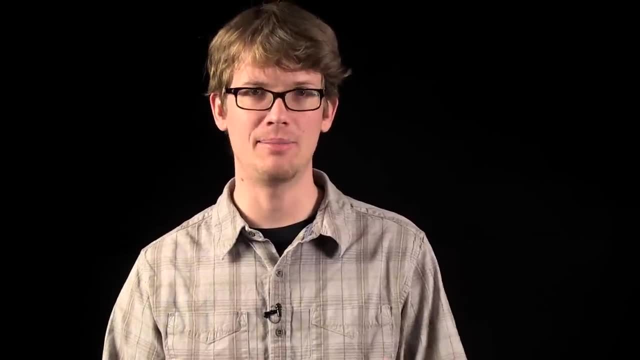 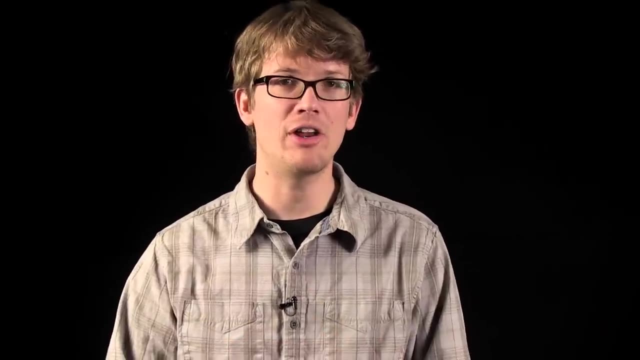 Now that we know the basics of DNA structure, we need to understand how it copies itself, because cells are constantly dividing and that requires a complete copy of all that DNA information. It turns out that our cells are extremely good at this. Our cells can create the equivalent of 10,000 copies. 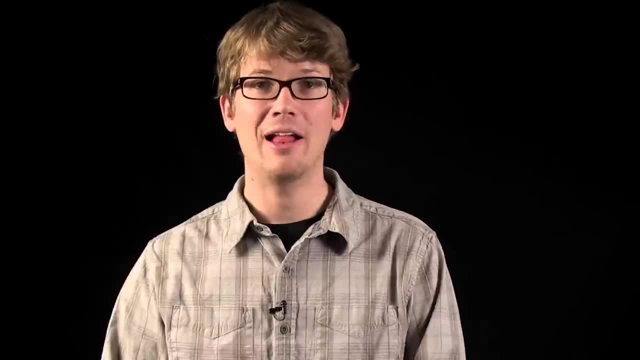 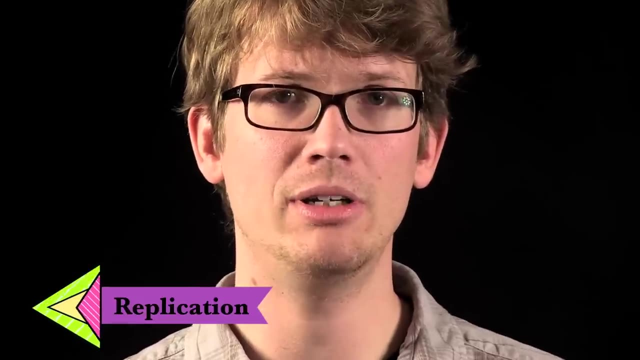 of this book in just a few hours. That, my friends, is called replication. Every cell in your body has a copy of the same DNA. It started from an original copy and will copy itself trillions of times over the course of a lifetime. 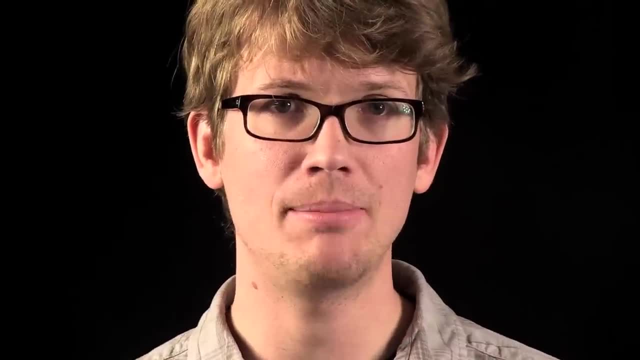 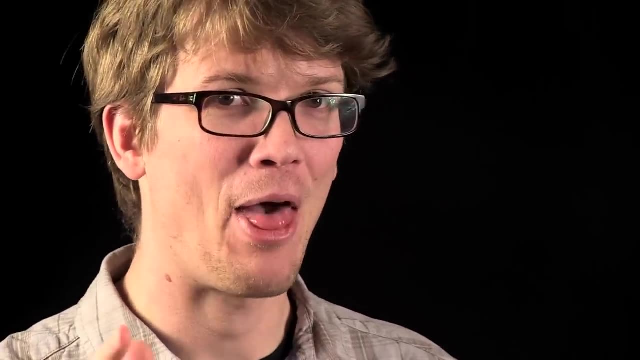 each time using half of the original DNA structure. Each strand is a template to build a new molecule. So how is a teenage boy like the enzyme helicase? They both want to unzip your jeans. Helicase is marvelous, unwinding the double helix at breakneck speed. 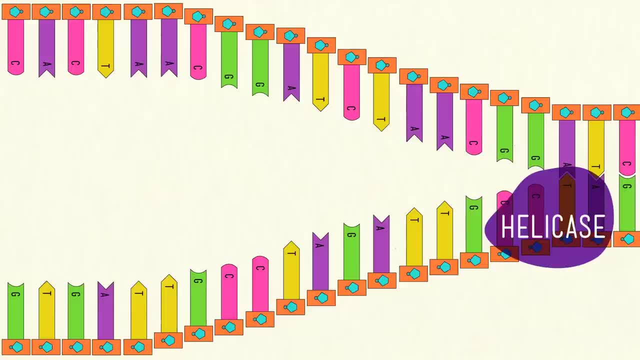 slicing open those loose hydrogen bonds between the base pairs. The point where the splitting starts is known as the replication fork. It has a top strand called the leading strand, or the good guy strand, as I call it, another bottom strand called the lagging strand. 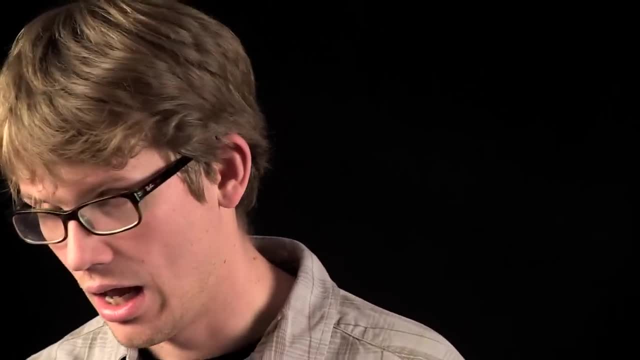 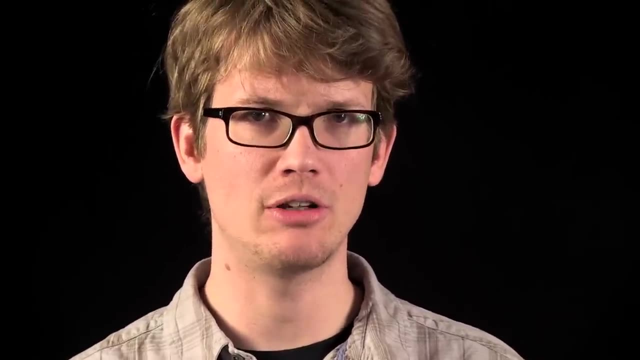 which I like to call the scumbag strand, because it is a pain in the butt to deal with. These unwound sections can now be used as templates to create two complementary DNA strands. but remember, the two strands go in opposite directions in terms of their chemical structure. 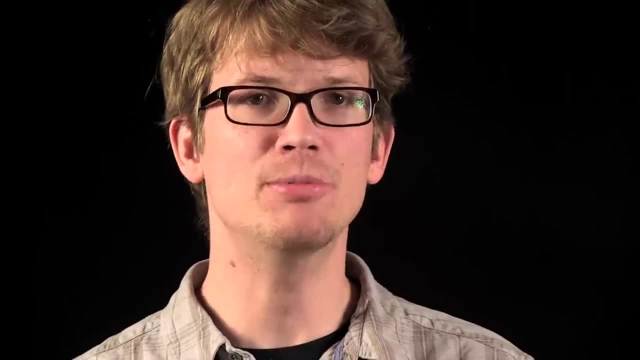 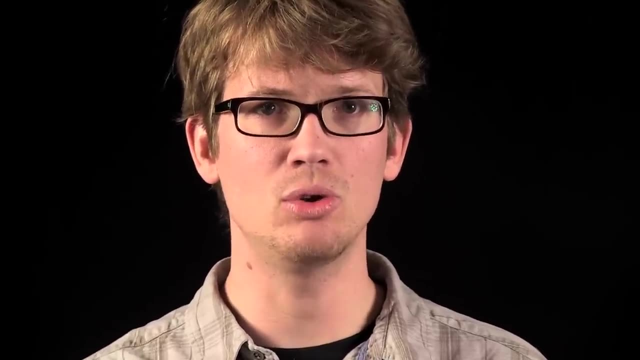 which means that making a new DNA strand for the leading strand is going to be much, much easier than for the lagging strand. For the leading good guy strand, an enzyme called DNA polymerase just adds matching nucleotides onto the main stem all the way down the molecule. 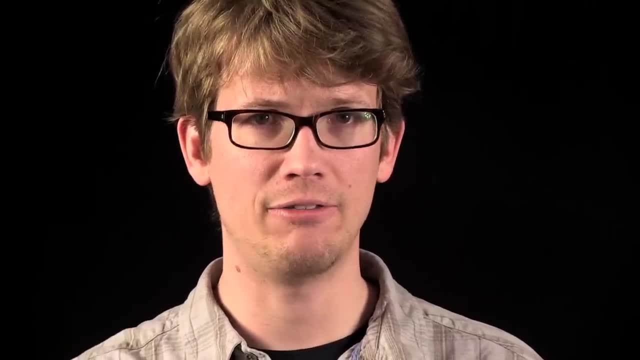 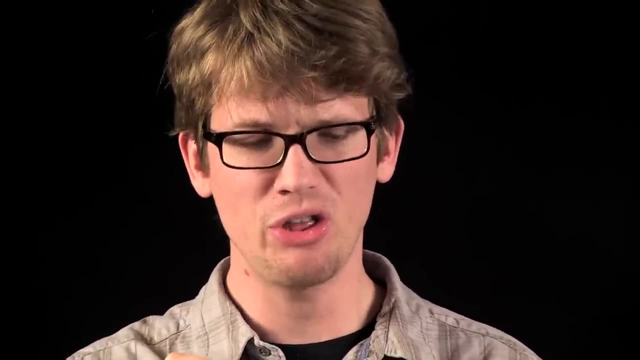 But before it can do that it needs a selection of nucleotides that fill in the section that's just been unzipped. To get started, at the very beginning of the DNA molecule, DNA polymerase needs a bit of a primer, just a little thing for it to hook onto. 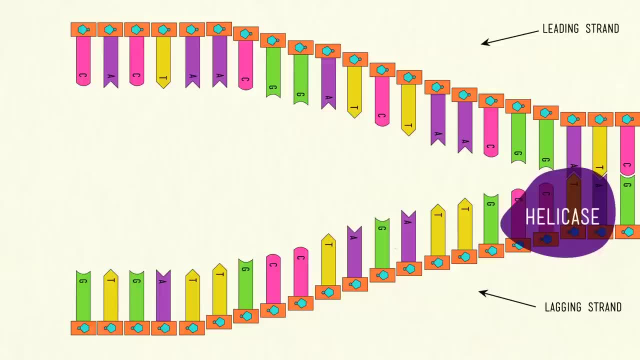 so that it can start building the new DNA chain. And for that little primer you can thank the enzyme RNA primase. The leading strand only needs this RNA primer once, at the very beginning, then DNA polymerase is all I got this. 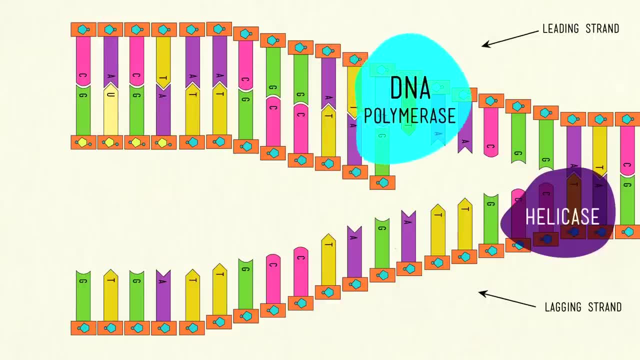 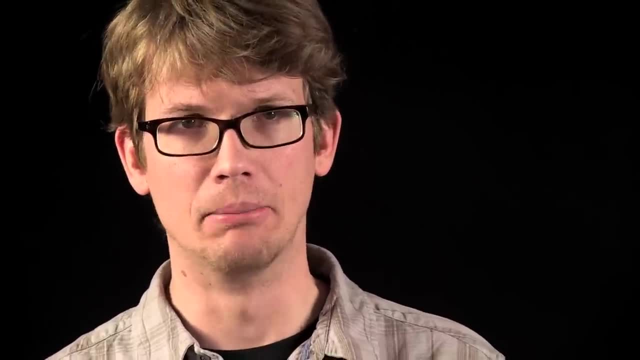 and it just follows the unzipping, adding new nucleotides to the chain continuously, all the way down the molecule. Copying the lagging or scumbag strand is well, it's a frickin' scumbag. 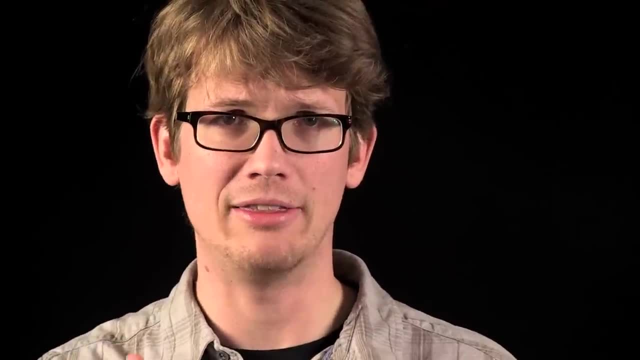 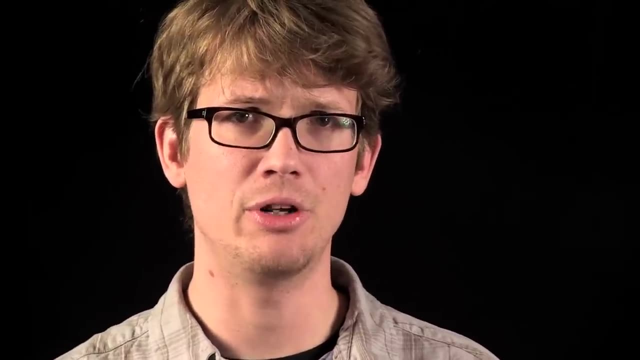 This is because DNA polymerase can only copy strands in the 5'-3' direction and the lagging strand is 3'-5', So DNA polymerase can only add new nucleotides to the free 3' end of a primer. 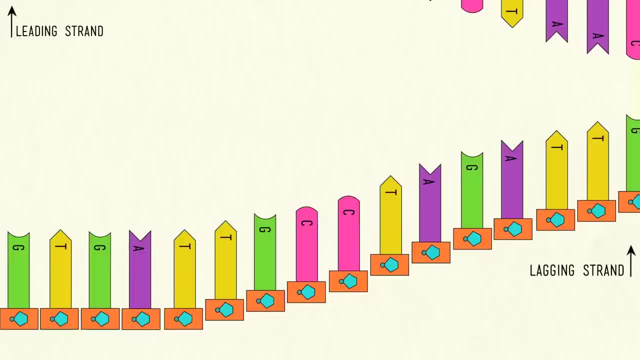 so maybe the real scumbag here is the DNA polymerase. Since the lagging strand runs in the opposite direction, it has to be copied in a series of segments, And here that awesome little enzyme, RNA primase, does its thing again, laying down an occasional short little RNA primer. 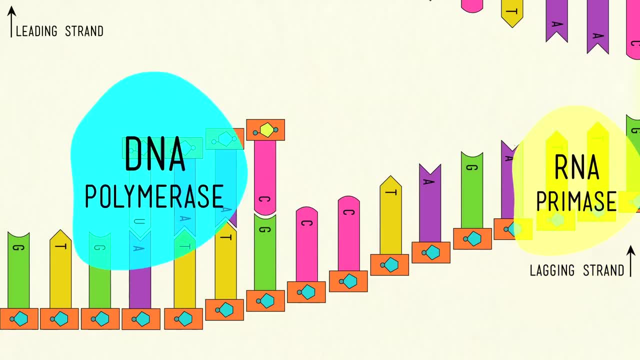 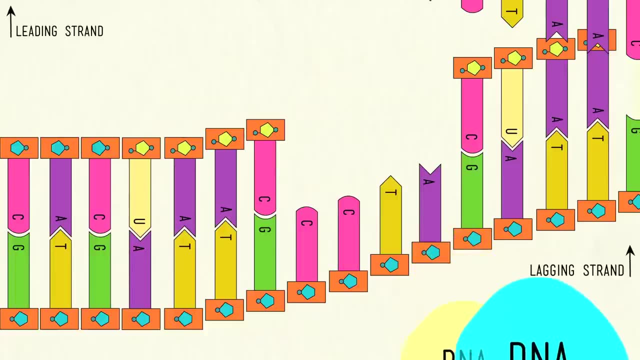 that gives the DNA polymerase a starting point to then work backwards along the strand. This is done in a ton of individual segments, each 1,000 to 2,000 base pairs long, each starting with an RNA primer. These are called Okazaki fragments. 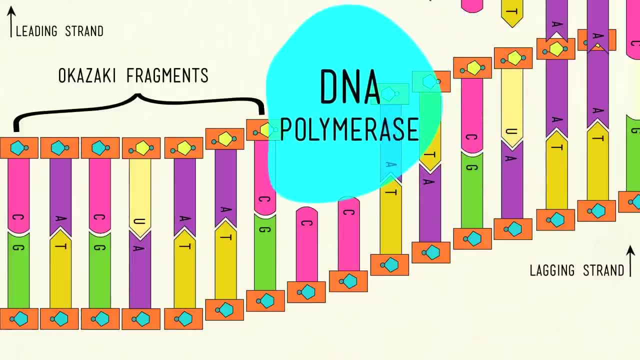 After the couple of married scientists who discovered this step in the process in the 1960s- and thank goodness they were married, so that we could just call them Okazaki fragments instead of Okazaki hyphen- someone's hyphen, someone fragments. 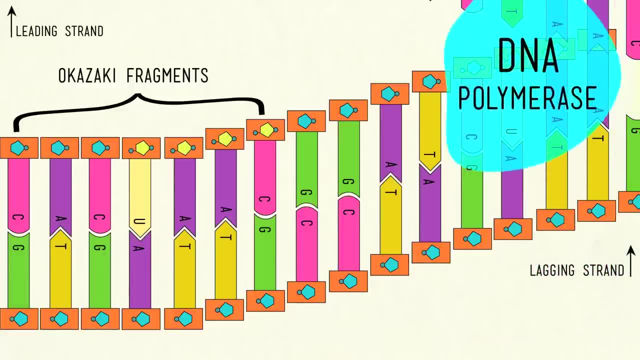 These allow the strands to be synthesized in short bursts, and then another kind of DNA polymerase has to go back over and replace all of those RNA primers, and then the little fragment gets joined up by a final enzyme called DNA ligase. 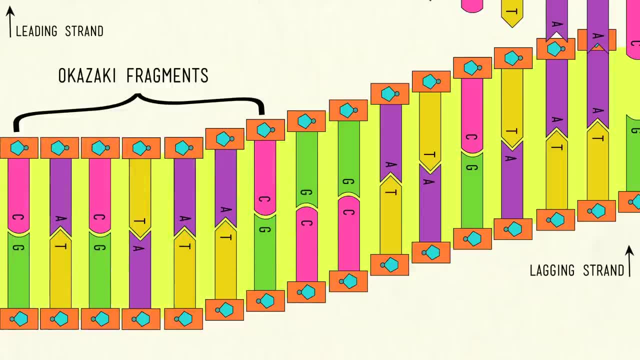 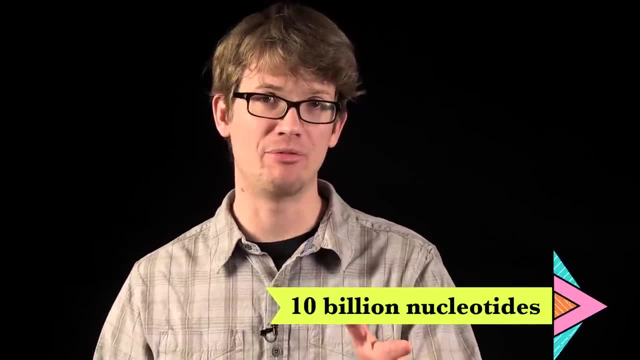 And that is why I say that the lagging strand is such a scumbag. DNA replication gets it wrong about one in every 10 billion nucleotides. but don't think your body doesn't have an app for that. It turns out that DNA polymerases can also proofread. 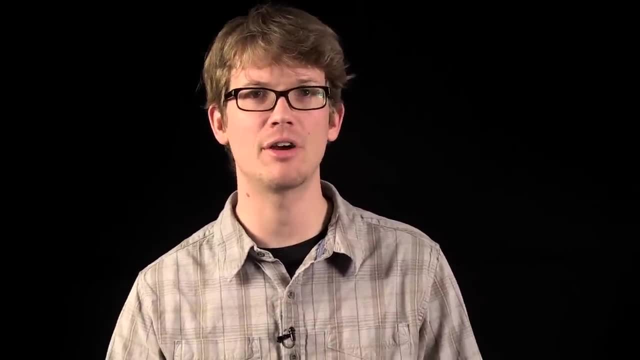 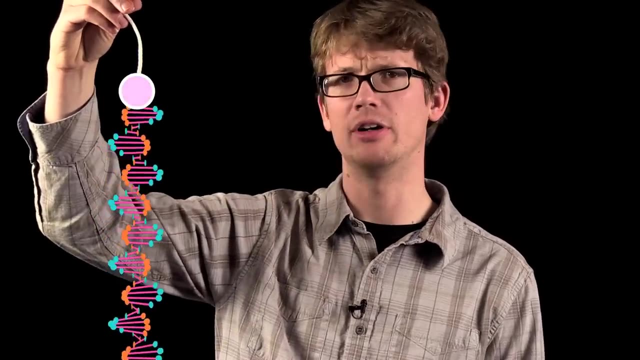 in a sense, removing nucleotides from the end of a strand whenever they discover a mismatched base, Because the last thing we want is an A when it would have been a G, Considering how tightly packed DNA is into each one of our cells.